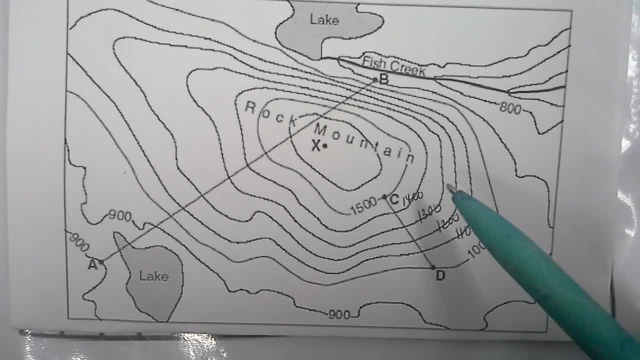 okay. so, having a look at how to actually do a cross-section, we need to have a look at point A, have a look at point B and we need to look at every single contour line along. so you need to take a piece of scrap paper and you need to mark. 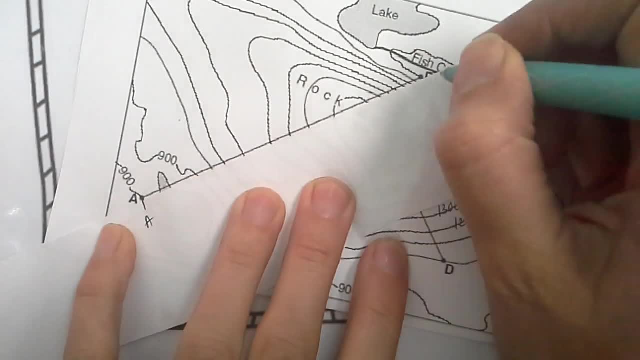 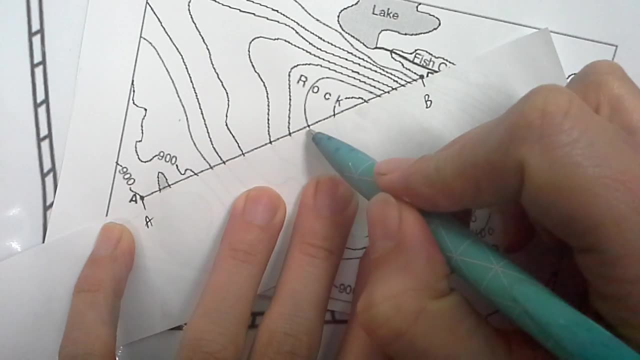 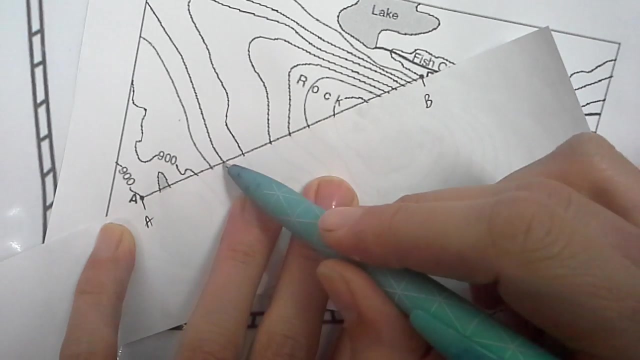 point A and you need to mark point B. so your job now is to have a look at every single contour line that crosses over where your cross-section is going to be. so this line, from A to B, every point along that line you need to be marking on your little piece of scrap. 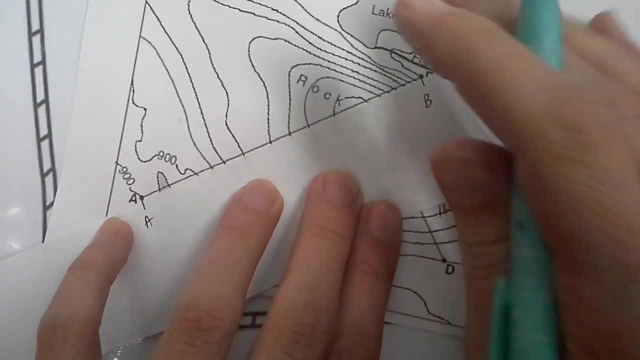 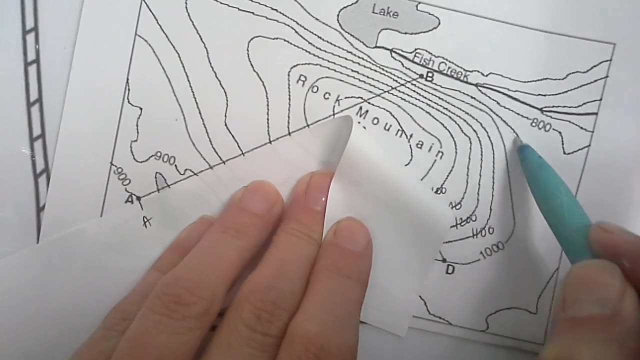 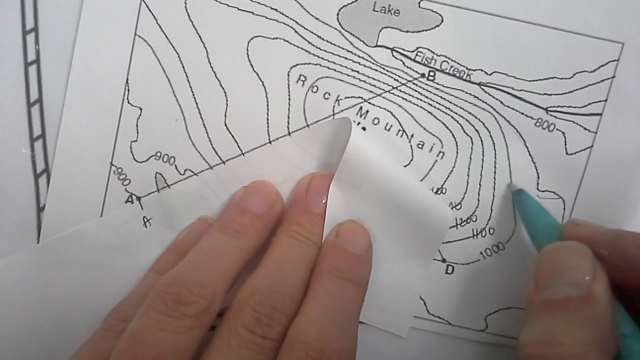 paper and we are going to use that information to create our cross-section. So we know that point B is over here, this line, and we know that that's a thousand, so we know that point B, then, is going to be a hundred, because the difference between the 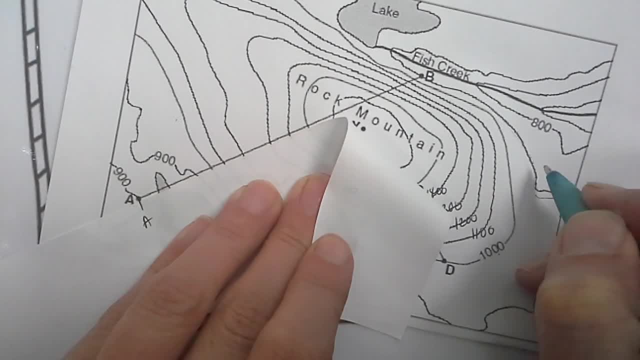 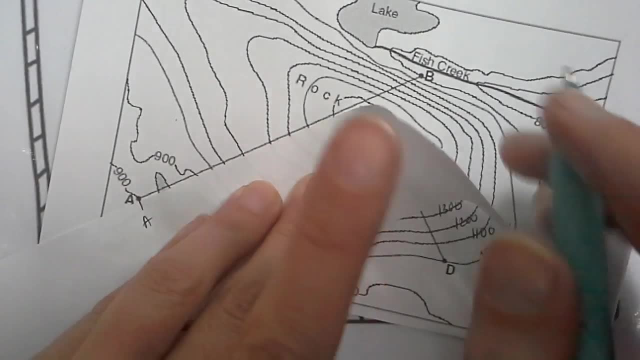 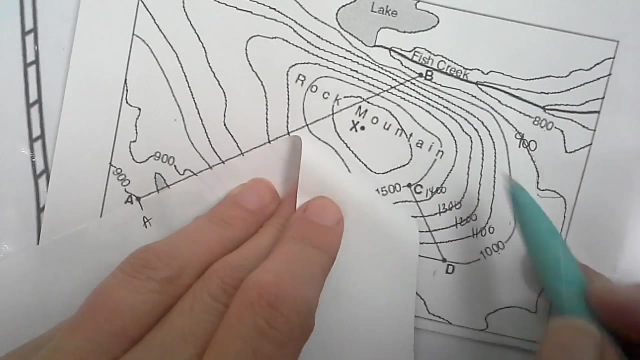 lines is a hundred meters, and so this is going to be nine hundred, because the difference between eight hundred and a thousand is nine hundred. so that makes perfect sense. So point B is nine hundred meters and we'e starting to climb up toward the mountain, So we've got 800, 900, 1000, 1100, 1200,, 1300,. 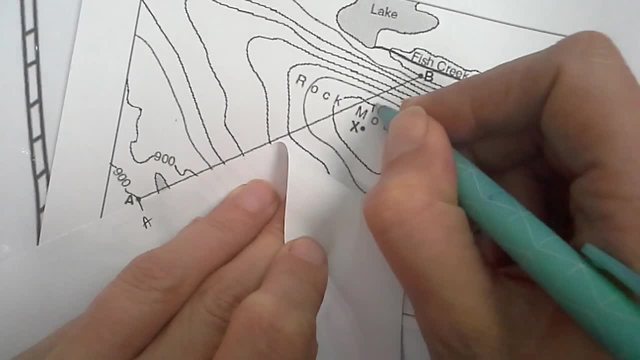 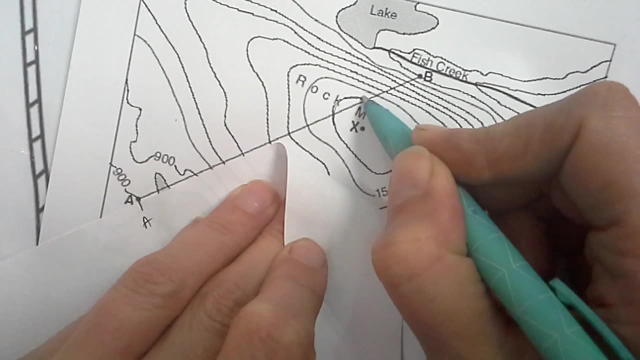 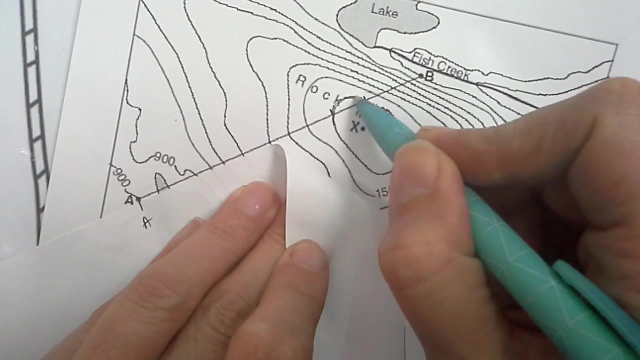 1400, 1500, and that will make this one here 1600. Because this connects. we can see that's all along the same contour line. it intercepts our cross section here at this section and also at this section. Now, both of these are along that same contour line, which is 1600. 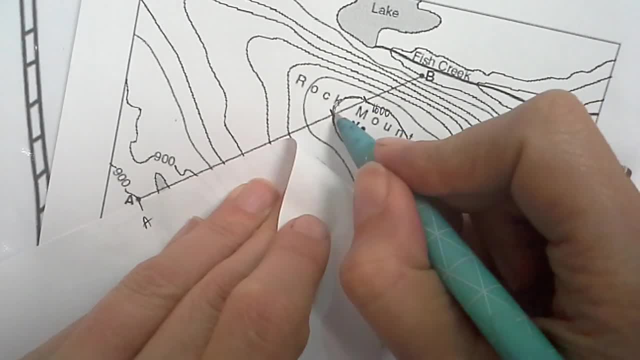 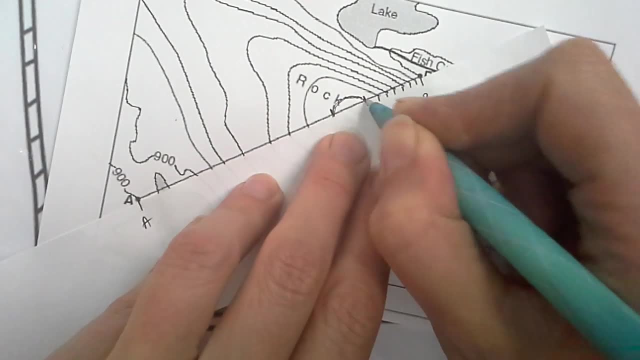 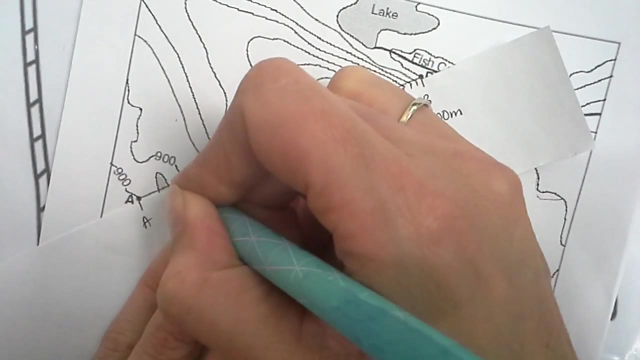 metres above sea level. So when we come to that one, they're both going to be identical. So let's go through now and mark each of these exactly as you see them in exactly the same spot along on your graph. Now you can write in the heights as you do that, or you can do. 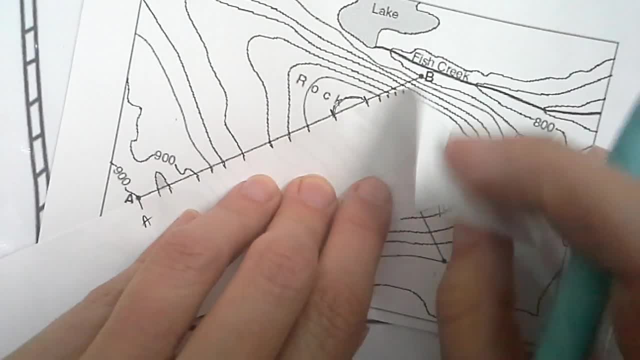 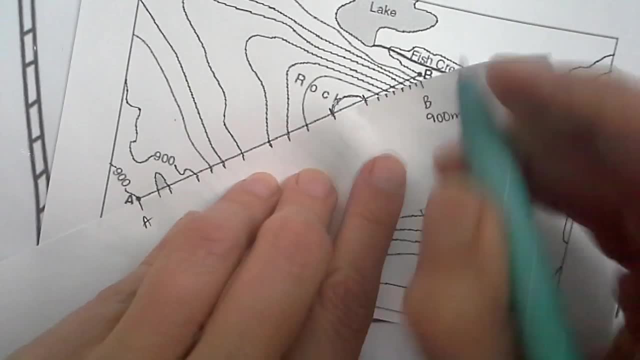 it afterward, depending on what you would like to do. So, having a look, here we've got 900, and then this one. here you can see all the way along we follow it- We have 1000. so that's this point here, and we know that each one of these represents. 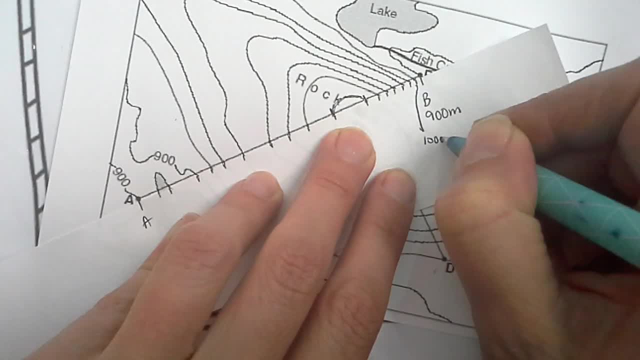 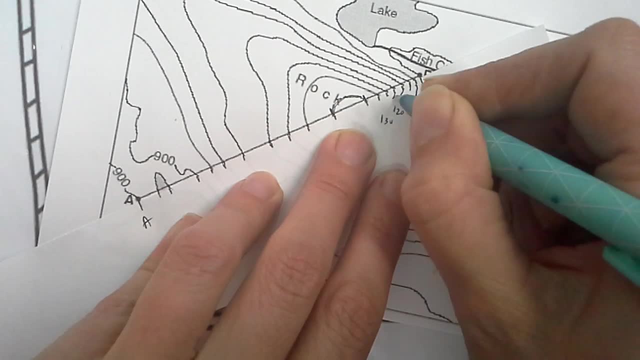 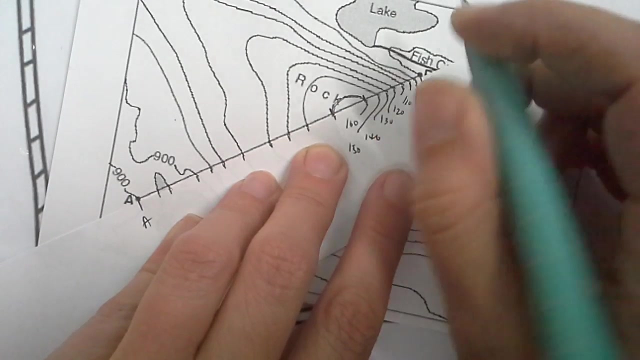 the same contour interval of 100 metres, so we've got 900 meters for 1000, which makes this 110, 120, 130, 140,, 150, 160 – well, I should actually do it properly, shouldn't I? 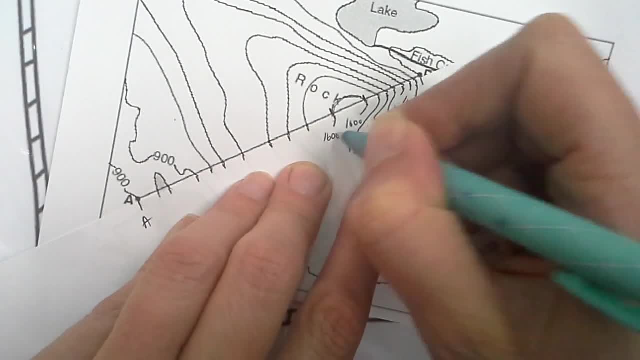 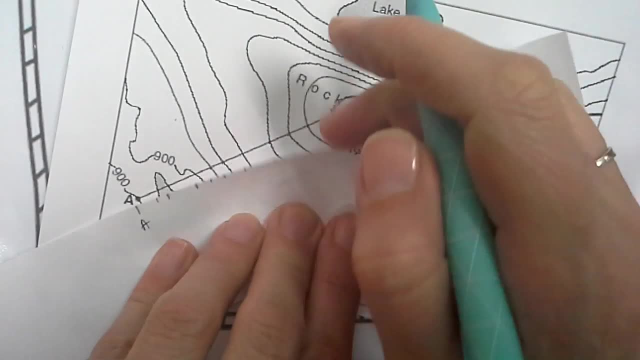 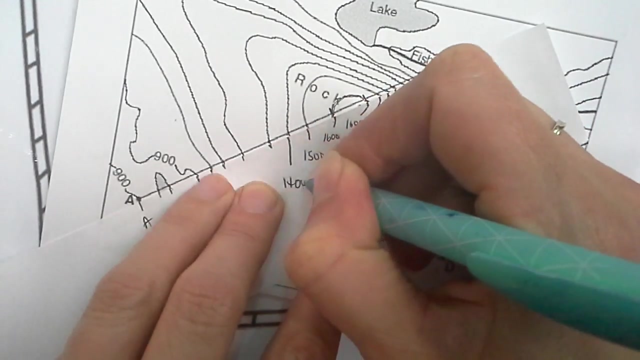 off the last zero. okay, so this is also sixteen hundred. and then we start on this side to start dropping off. so we can see down here it's nine hundred and we're building up toward the top of that mountain. so we've got sixteen hundred, sixteen hundred. this one becomes fifteen hundred, fourteen hundred thirteen. 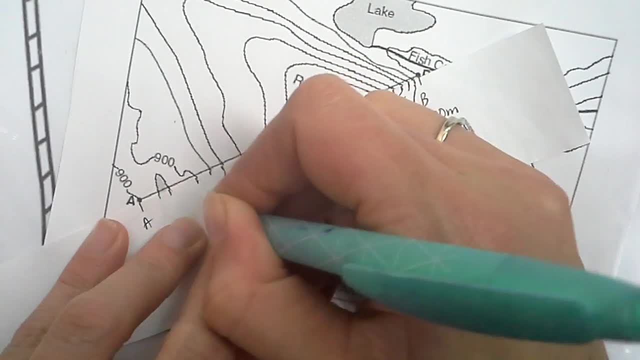 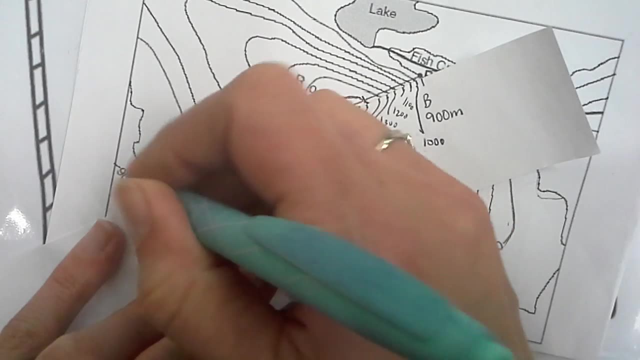 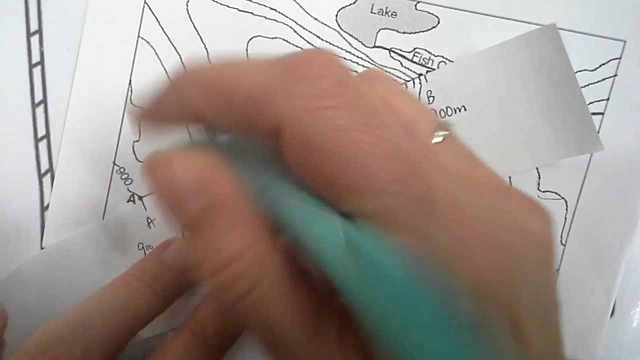 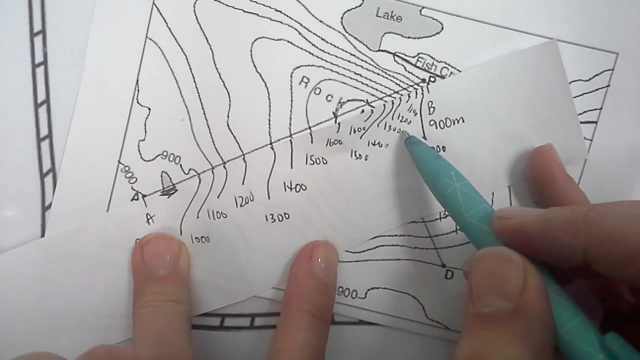 hundred twelve eleven, ten, well, ten hundred a thousand nine hundred, and this point here is also nine hundred. so, having a look here, that's just a lake. we're going to disregard it. we don't need to know that for grade eight geography. okay, so you can see, it's a lot easier to write in up this end. it's a. 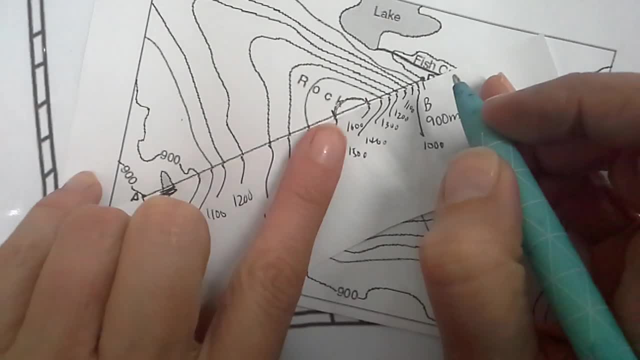 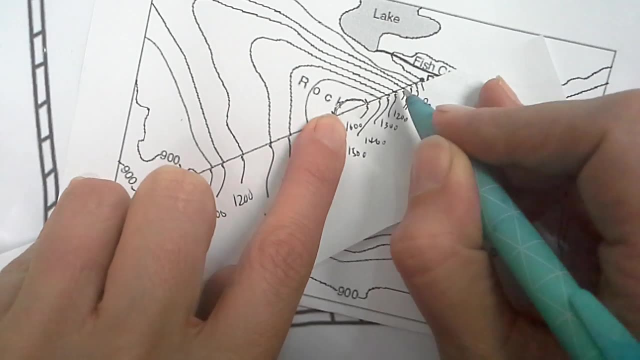 lot more squishy putting your numbers in. so the main point is that your line is going to be a little bit smaller and then you're going to have a little bit more line intersects exactly where that comes along the line here. okay, if that's off, then your whole cross sections going to be off. so as long as your point. 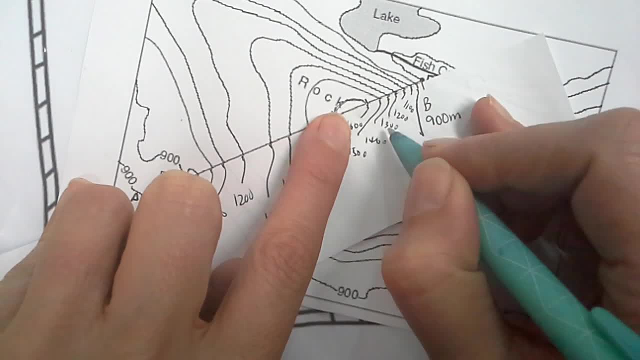 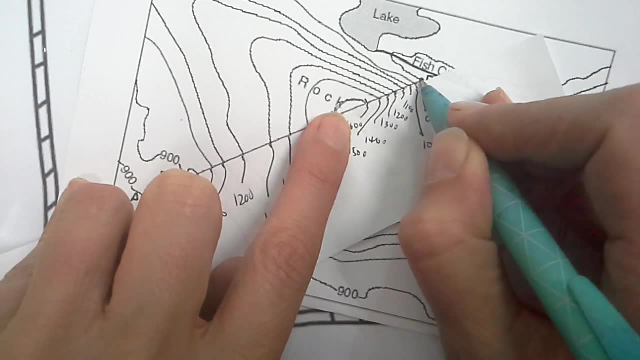 starts where it needs, at the top of the page. you can draw a line down here and write 1,300- where you've got a bit more room- okay, but as long as it matches up with the lines directly along this section here, okay, so we've got all of. 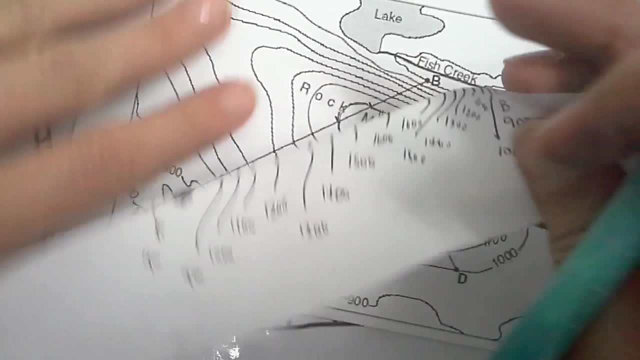 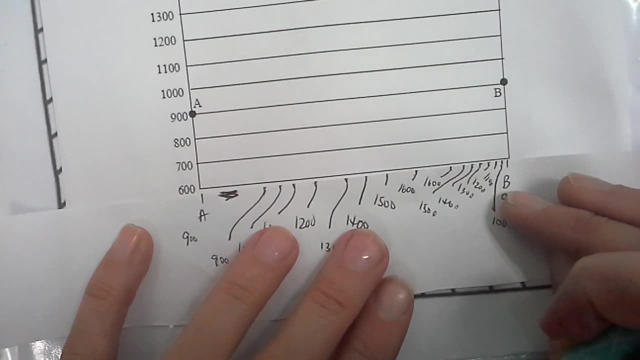 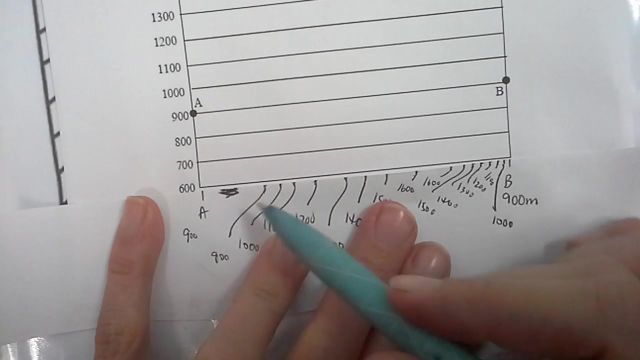 our measurements in now and we've got them all mapped on here. we're going to look at plotting them now on this map. so this one has already been done for us, which is excellent. but if we have a look here, the width of your graph down here is only ever going to be the width of the points. 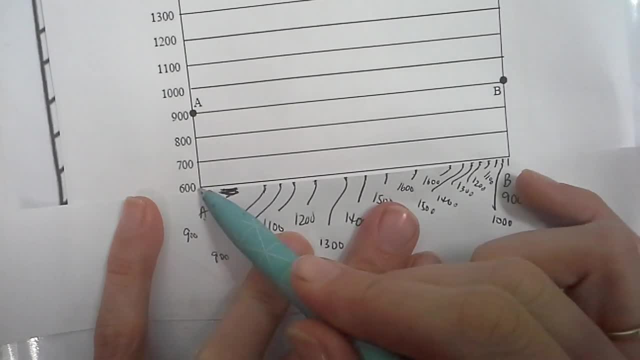 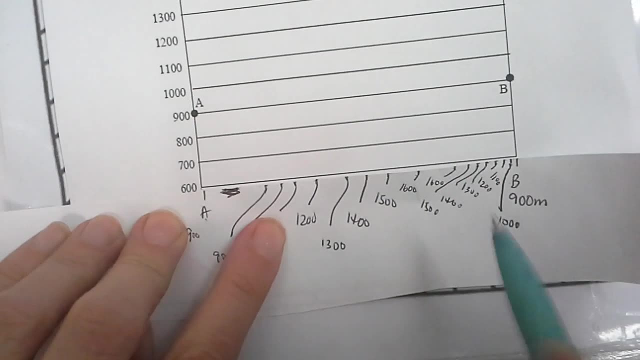 that you're actually going to be mapping. so A to B, it's beginning to finish. okay, if your cross-section is only this small, then your graph that you're plotting it against it will only be that small as well. all right, so there's no need to. 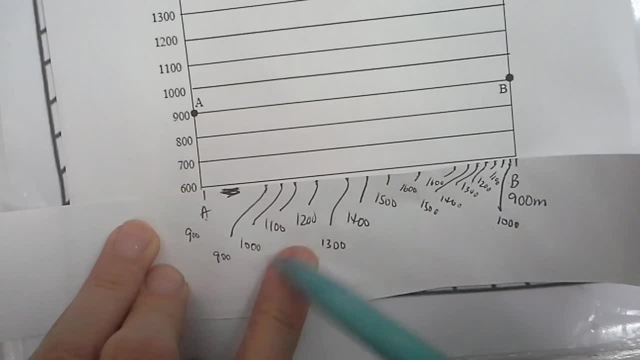 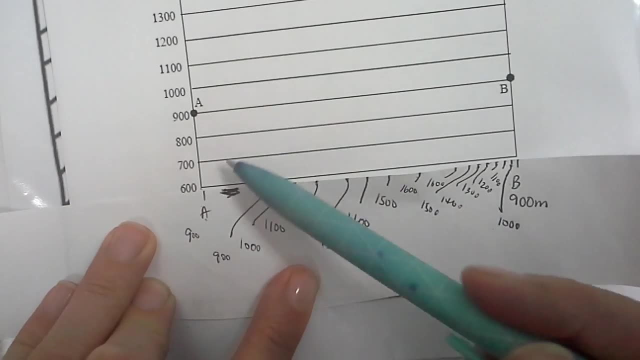 have a big, giant long one if your cross-section is a lot smaller than that. now, looking at this axis, we can see that goes from 600 to 1700, all right, and so that's a pretty broad range. the main thing that you want to make sure is see. 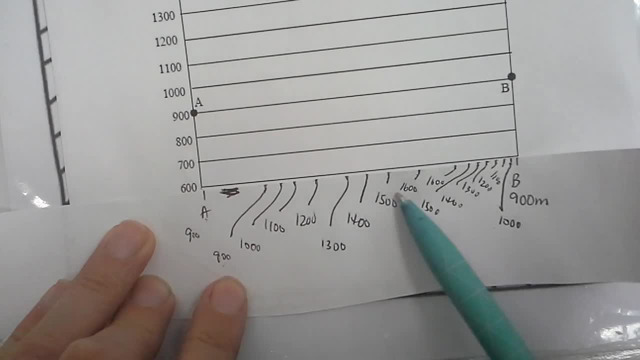 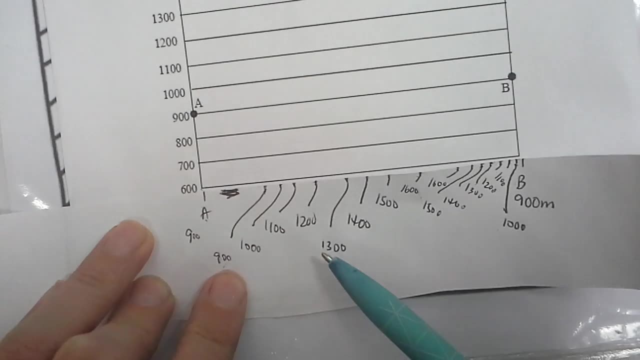 my smallest one here is 900 and my biggest one is 1600, so as long as I've got a range up this side from 900 to 1600, it's going to fit my cross-section. this one's a bit broader and that's fine as well. okay, so having a look. the next. 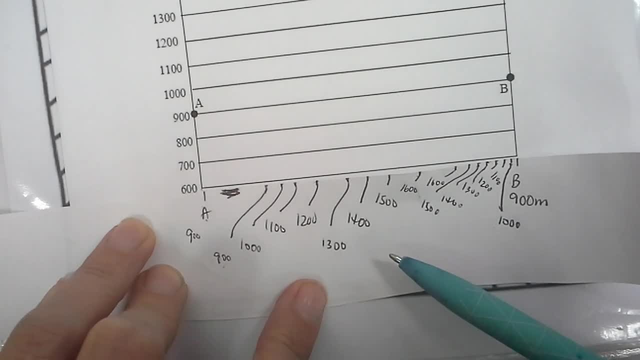 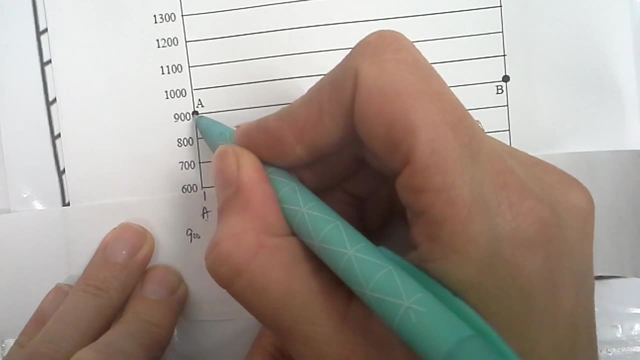 thing to do- and this is one of the most important tasks- to make sure that you're getting the right shape. okay, we've got point A labeled on there and that's already in here for us, luckily, so point A is at 900 meters. now the next dot. 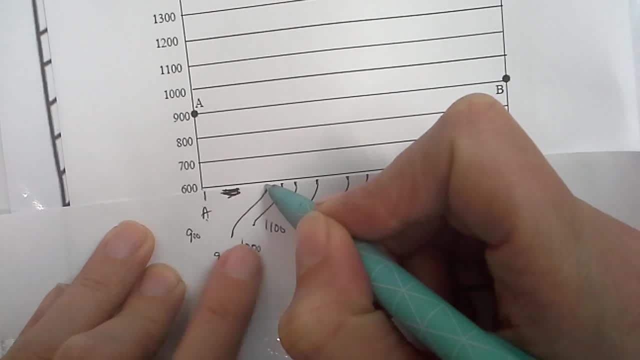 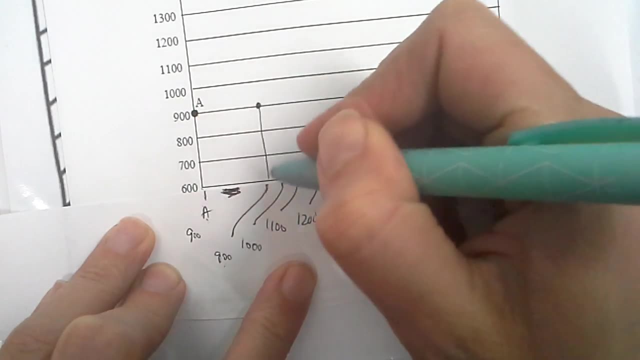 point that we're going to do is going to line up directly with where we put that line on the page. and again, we're coming all the way up and we're looking at bang 900. okay, you don't need to draw that line in, but you do need to make sure it's. 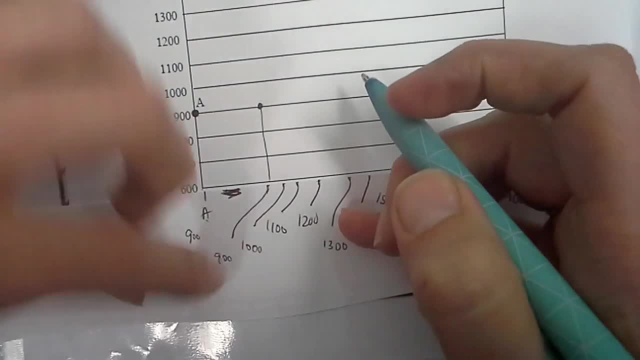 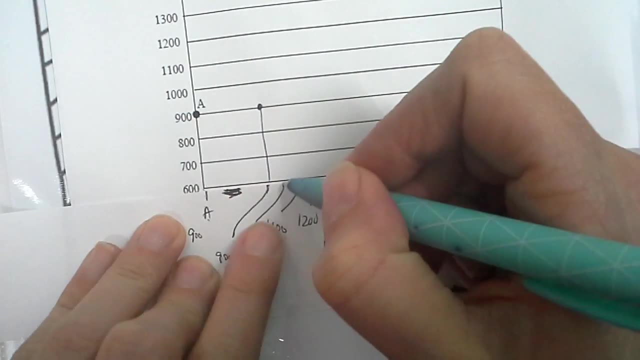 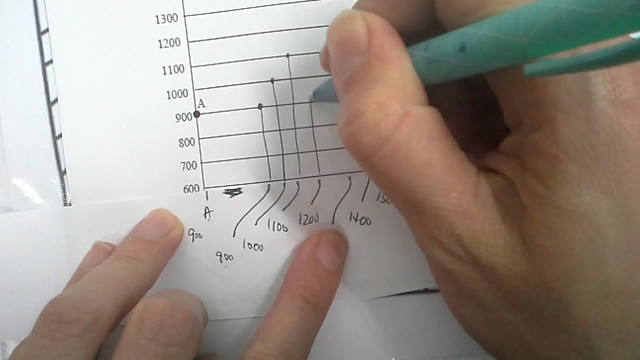 straight. so some people like to take a ruler and they use that along this way to line up that with where it needs to be along this axis of the graph. okay, so this one here is a thousand eleven hundred twelve hundred, and you're doing this very neatly. grade eight: you're not scribbling like I am, and 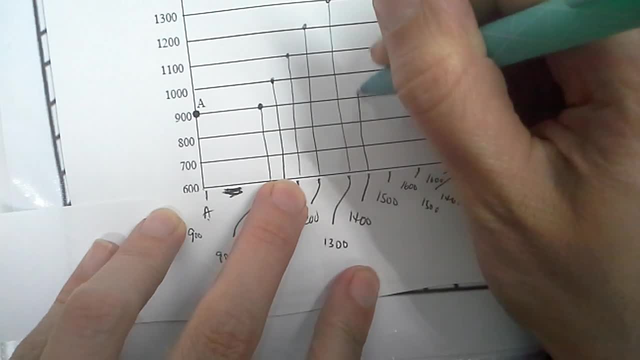 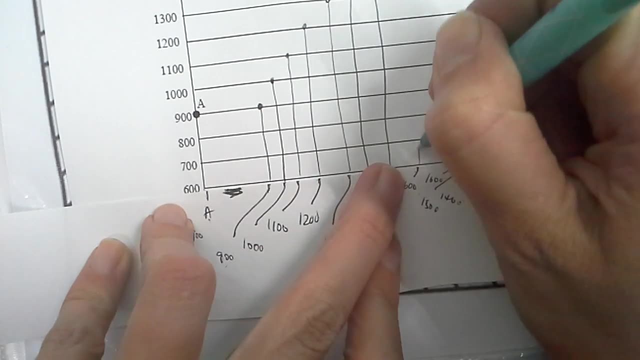 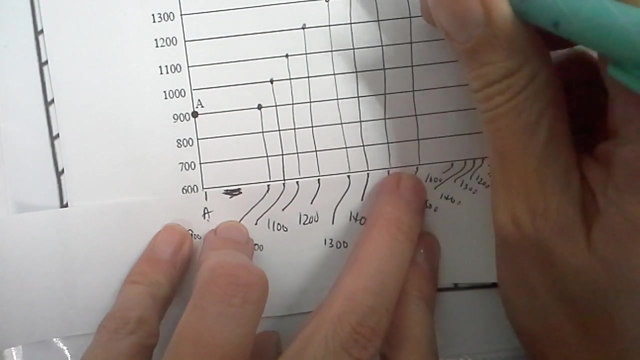 you're probably doing it in pencil too, in case you get anything wrong. okay, fourteen hundred is here, all the way up to fifteen hundred sixteen hundred, and these again are perfectly lined up directly with that point. see, that's a little off. that's wrong. you're going to do it very. 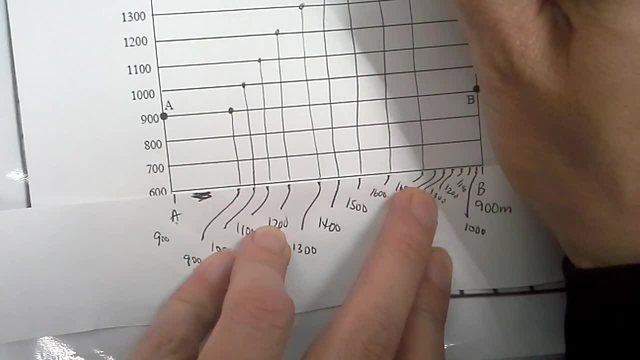 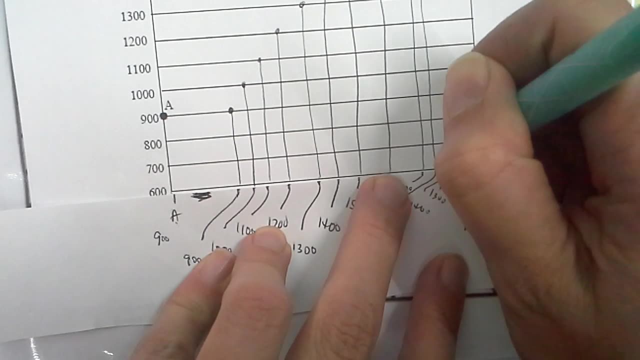 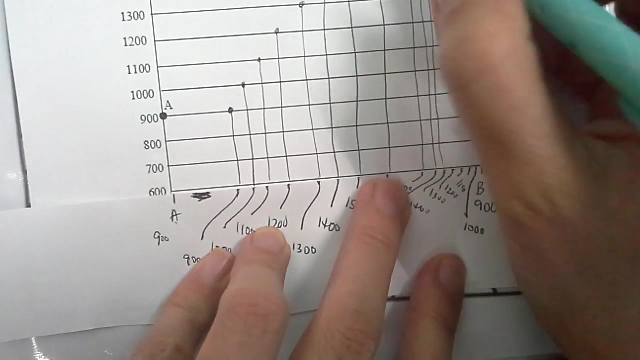 neatly again. sixteen hundred fifteen hundred fourteen, and you can see they're starting to get a lot closer together and you can see, instead of this gentle slope with them, a bit further apart it's starting to come down really quite heavily because the lines are closer together, the contour lines. all right.